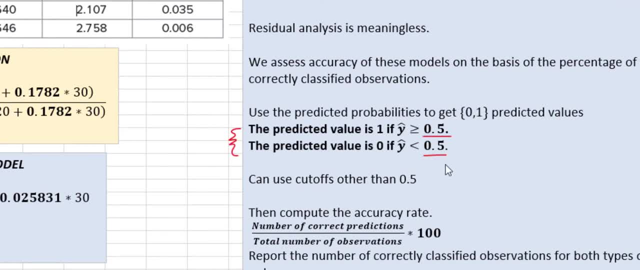 value. In many analysis the cutoff value of 0.5 is used. So what does that mean? That means the predicted value is equal to 1 if the predicted probability is greater than and equal to 0.5, and the predicted value is going to be 0 if the predicted probability is less than 0.5. Then the 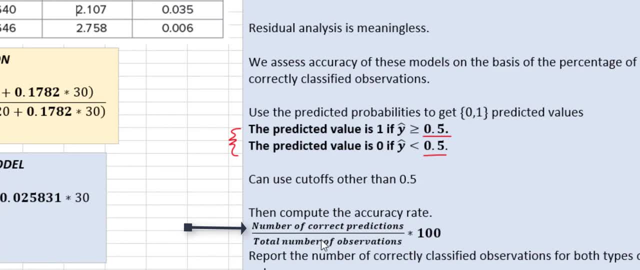 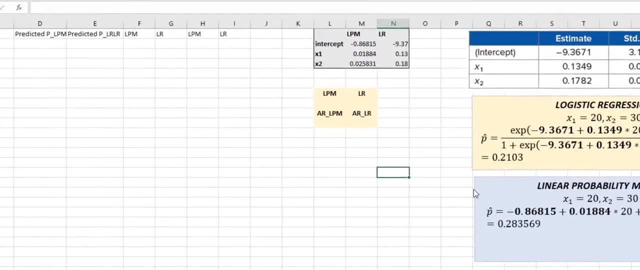 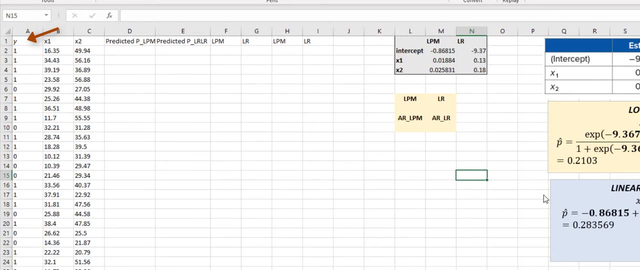 accuracy rate is calculated as the number of correct predictions divided by the total number of observations times 100.. Here in this video we continue to analyze mortgage data. Recall that in mortgage data, y represents loan approval and y is 1 if the loan is approved and 0 otherwise. x1 is down payment and x2 is loan to value ratio. Both. 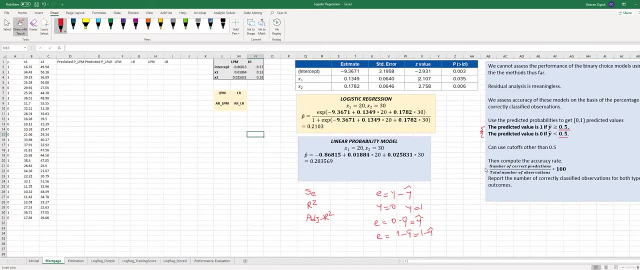 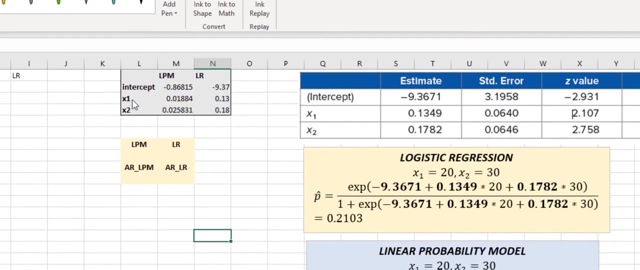 are in percentages. So to determine the accuracy rate we need to know the predicted probabilities. For linear probability model calculating p hat is based on the linear regression and regression parameters estimate. Here you can find the coefficient estimates from the linear regression intercept x1 and x2.. So predicted probability is: 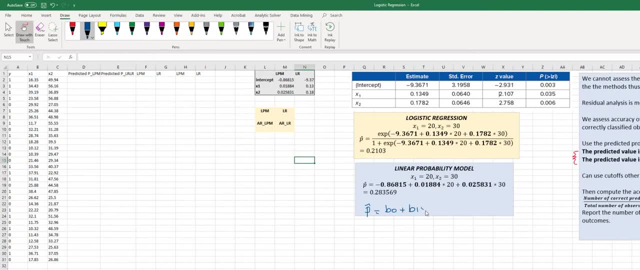 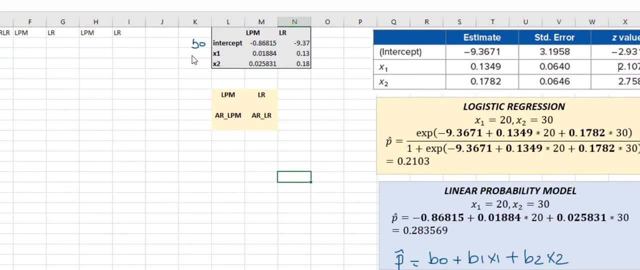 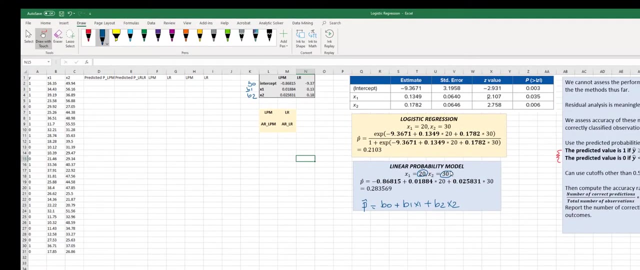 x1, b0 plus b1, x1 plus b2, x2.. Here in this table, b0 is here b1 and b2.. So let's say x1 is 20 and x2 is 30. Then the predicted probability is b0, which is negative, 0.86815, plus b1, which is 0.01884 times. 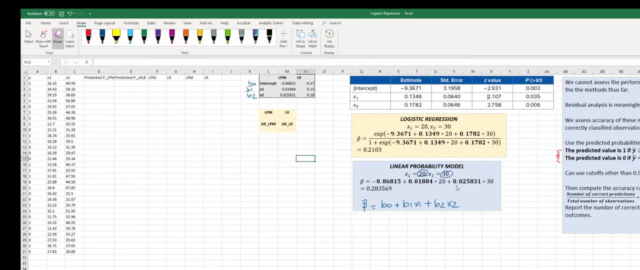 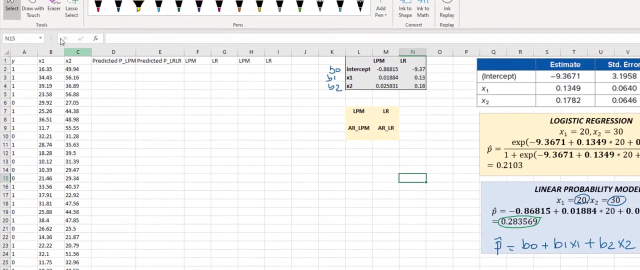 20x1 plus b2, which is 0.025831 times x2.. So the predicted probability is calculated as 0.283569.. And we are going to use this linear line to predict the probabilities for our data. Here we start with an equal sign and then select the intercept. We need to fix the values because 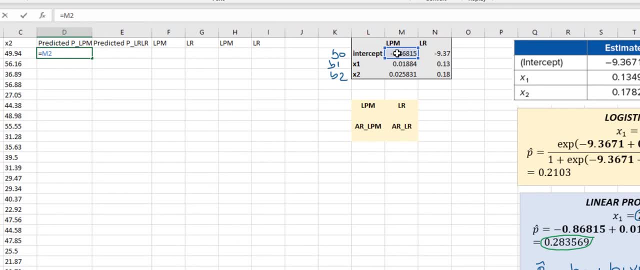 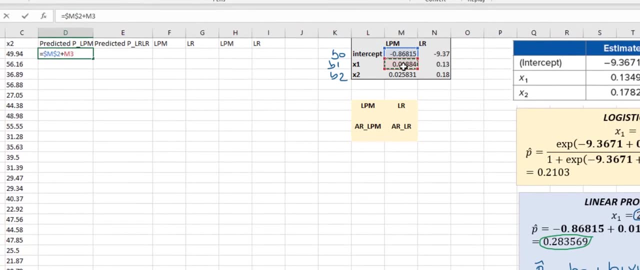 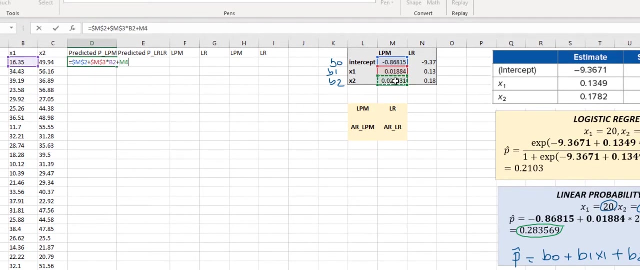 when we drag down the formula, we want to refer to the same intercept value. Therefore, click f4 and plus select b1, and then click f4 times x1, plus select b2, and we need to fix that again: f4 times x2 and then enter. This is the predicted probability for linear probability model. And now 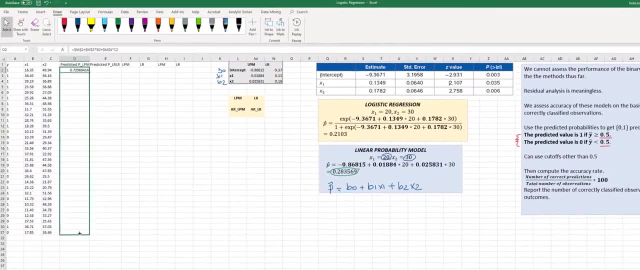 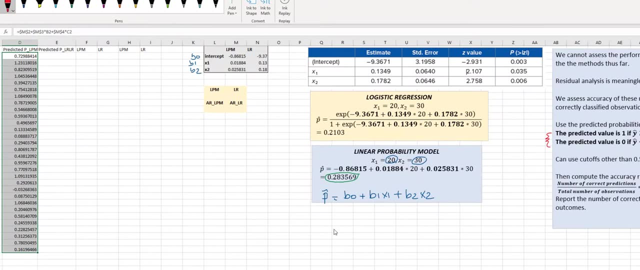 we drag down the formula to calculate for other x1 and x2 values. Now, next, we are going to calculate a development formula. Click the formula, click the isopropyl law, For example, for a single x0 and logistic regression, predicted probabilities. And if you recall from, 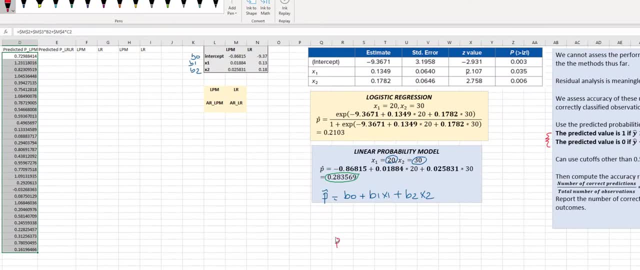 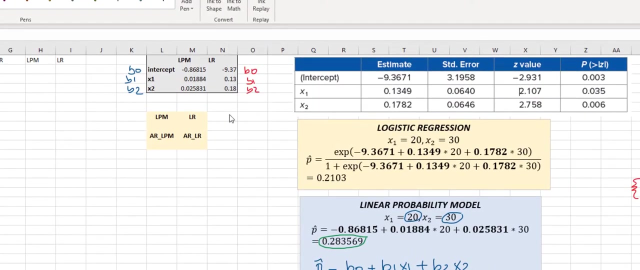 previous videos. logistic regression: predicted probability is found using the logistic specification. It starts with: e to the power b0 plus b1- x1 plus b2- x2, divided by 1 plus e to the power beta 0 plus b1- x1 plus b2- x2.. Here b0, b1, and b2. 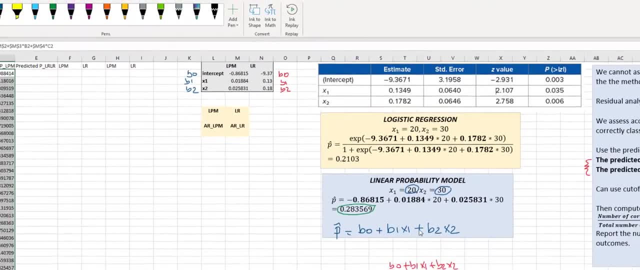 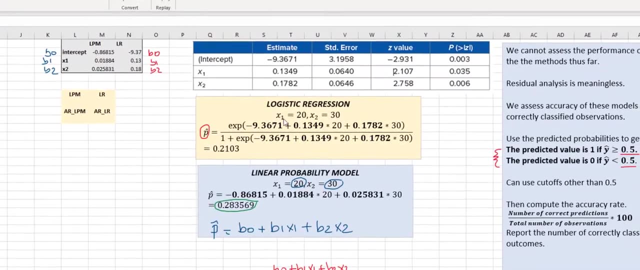 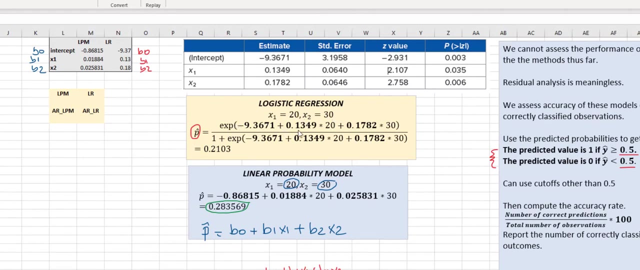 are already estimated. And now what we need to do is we need to plug the values in the formula. Let's say we want to predict the probability for x1 is equal to 20 and x2 is equal to 30. Then in the parentheses we have b0 plus b1 times 20. 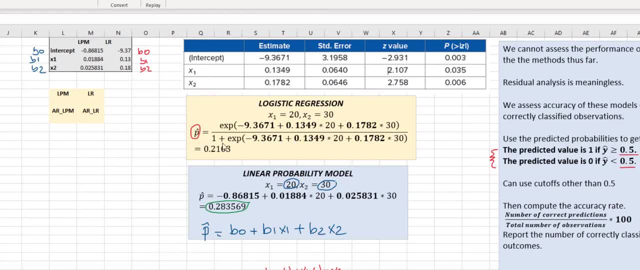 plus b2 times x2, divided by 1 plus exponential, And then in the parentheses you have the intercept b0 plus b2.. b1 times 20 plus b2 times x2.. When you calculate this equation, you find a predicted probability is 0.2103.. Now here we are going to use the same 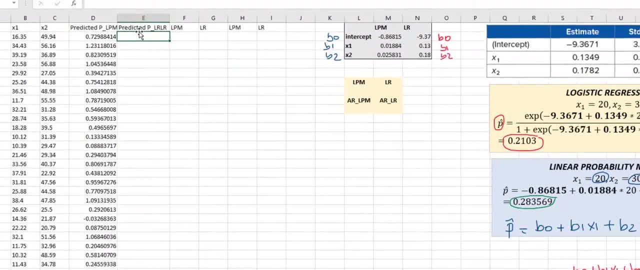 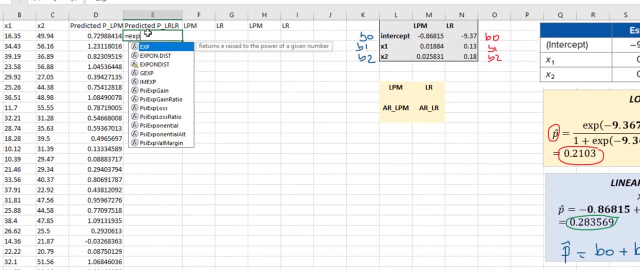 specification. to calculate the predicted probabilities for our sample, Start with an equal sign For exponential. there is a function in Excel called exp. Open the parentheses and now we are going to select the intercept, which is b0, and fix the value Plus b1.. Fix that value again And then times x1 plus b2.. Fix the value. 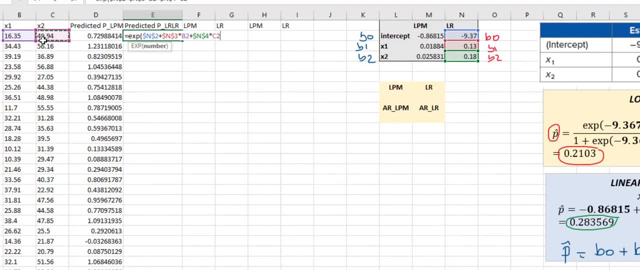 And then times x2.. Close the parentheses. And now for division. we use division. sign In parentheses 1 plus again exponential function. Open the parentheses b0.. Fix the value using f4.. b0 plus b1.. Fix the value Times x1 plus b2.. We fix the value first: Times x2.. Close. 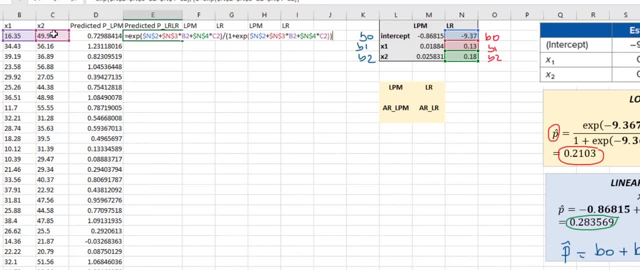 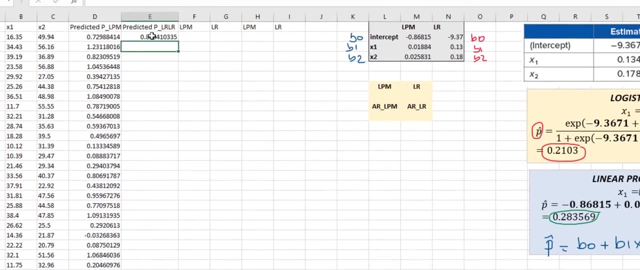 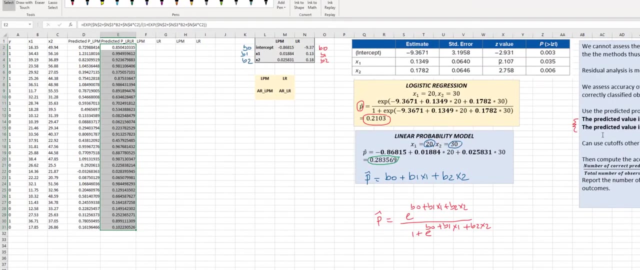 the parentheses for exponential function and close the parentheses second time And then click enter. Here this is the predicted probability of the first observation, using logistic regression model. Now we are going to drag down this formula. Now we are going to use the cut-off value 0.5 to determine whether the predicted value is going to. 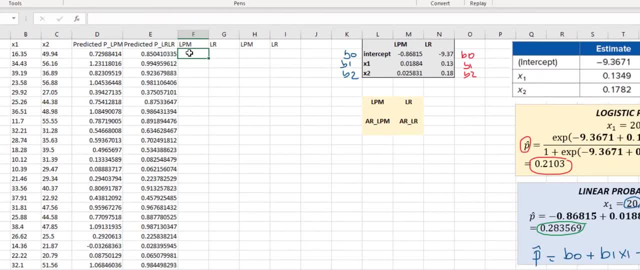 be 1 or 0.. Let's start with the linear probability model and we will use if function. If predicted probability for linear probability model is greater than equal to 0.5, the cut-off value, then the predicted value is 1, otherwise 0.. And close the parentheses and enter. Now we are going. 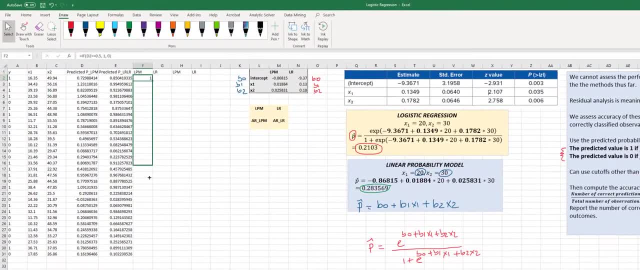 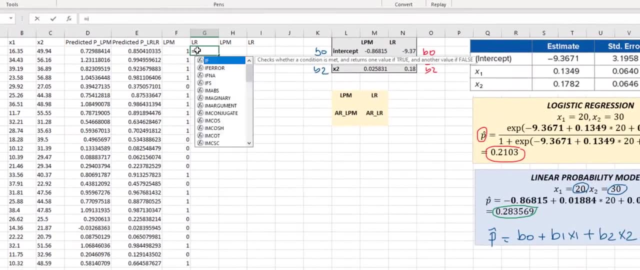 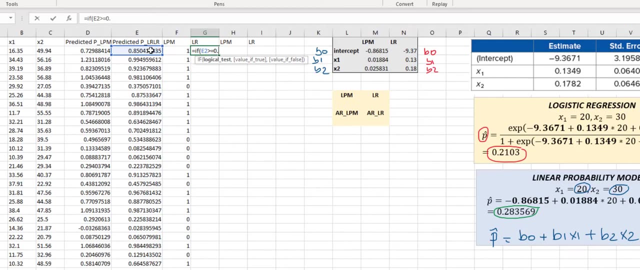 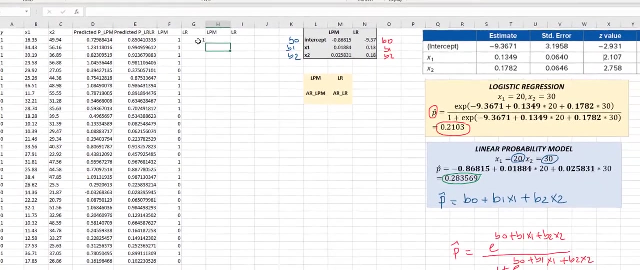 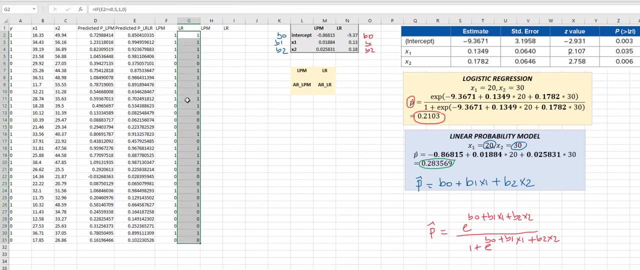 down the formula to find out the predicted values and we will repeat the steps for logistic regression if the predicted probability is greater than or equal to 0.5 than 1, otherwise 0, and close the parentheses and drag down the formula. so we calculate the predicted values. now we need to find out how many. 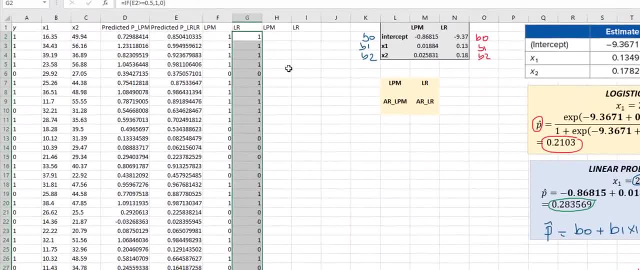 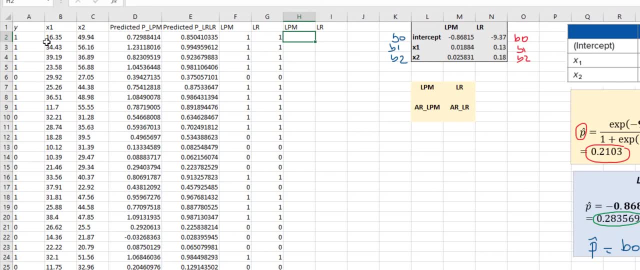 of these predicted values are actually correctly identified. to do that, we need to compare this predicted value with the actual value, and if the predicted value is the same as the actual value, then we need to count the number of predicted values that are correctly identified. this time we use again, if function, our 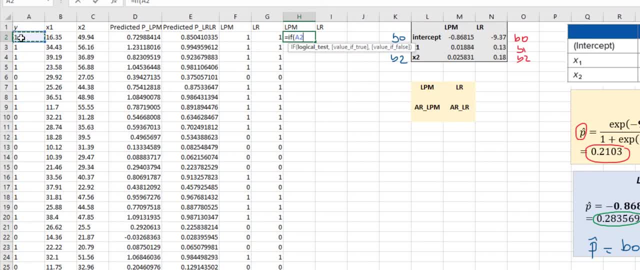 logistic regression is equal to 0.5 than 1. logical test is: if the actual value is equal to the predicted value, then type true, otherwise false, and close the parentheses. and, as you see, the first value is true because predicted value is 1 and the actual value is 1 too. and now, 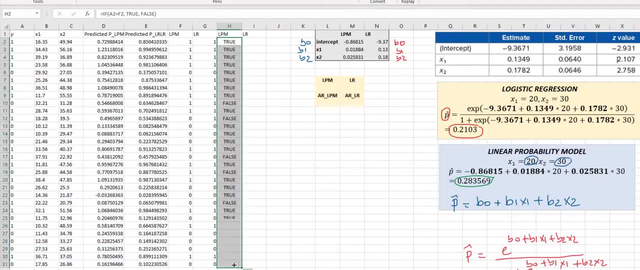 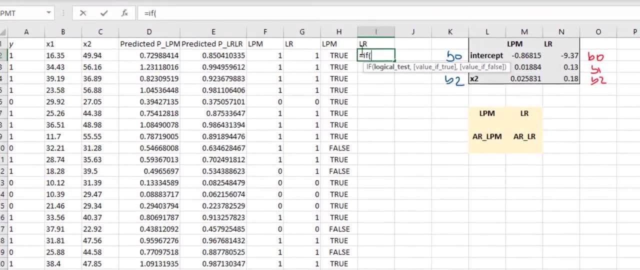 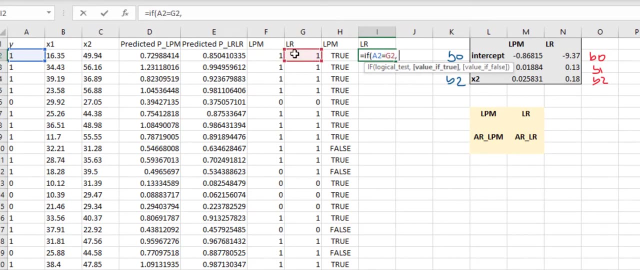 we drag down this formula and find out trues and false, and we will do the same thing for logistic regression. start with if and our statement is actual, equals the predicted value from logistic regression and if they are equal true, otherwise false, and close the parentheses and you can drag down this. 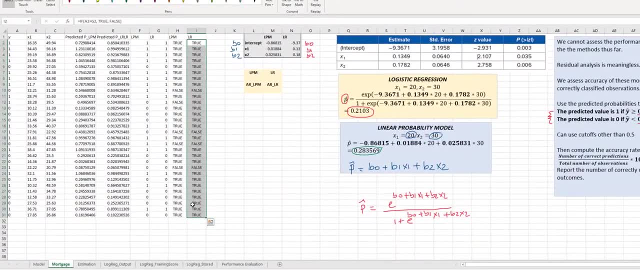 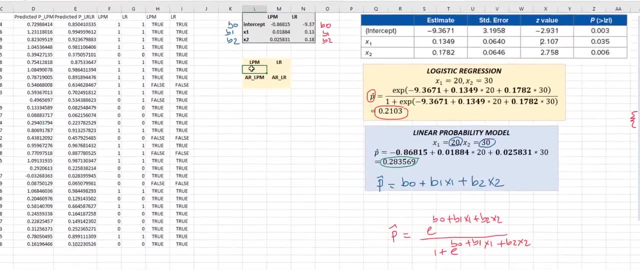 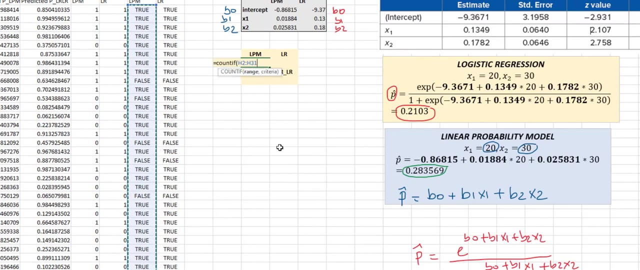 formula and now we have the trues and falses, but we want to count how many of them are correctly specified. therefore we will use here count if function. this time we are counting all true values in this column. here we select the column and count the true and, as you see, 25 observation out of 30. 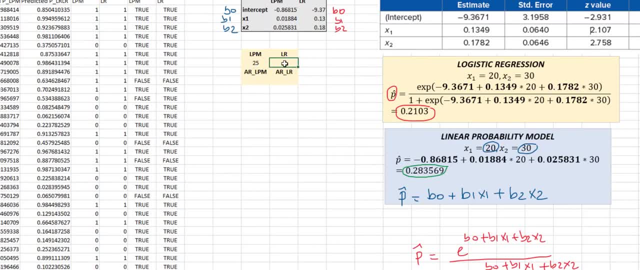 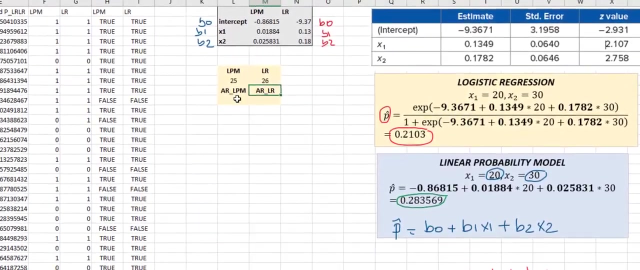 observations are correctly identified. now we will do the same thing for logistic regression: count if and open the parentheses and choose the range and then count the true values, close the parentheses and logistic regression correctly identifies 26 observations. and finally we will calculate the accuracy rate for linear. 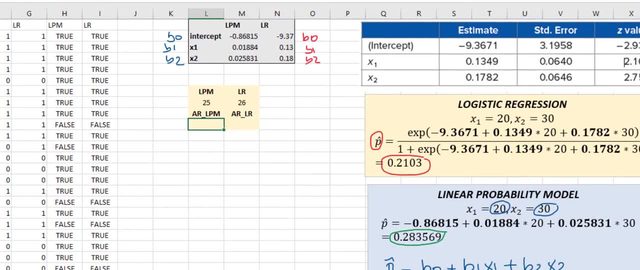 probability model. here we are going to calculate the number of correct predictions divided by total number of observations, and we know that we have total 30 observations. therefore, accuracy rate is equal to 25 divided by 30, and we will do this for logistic regression. we correctly identify. 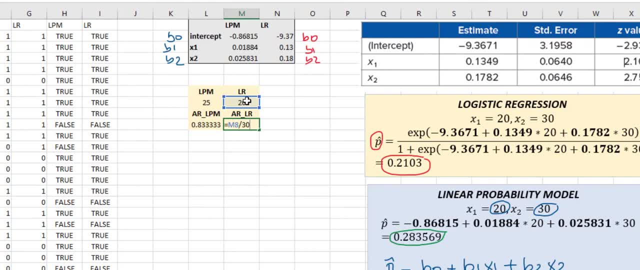 20, observation rating and closing iron goes to 5. we have 25 observations and this formula observations and the total number is 30, so the accuracy rate is 0.86667.. This is how we measure the performance of binary choice model Logistic regression. 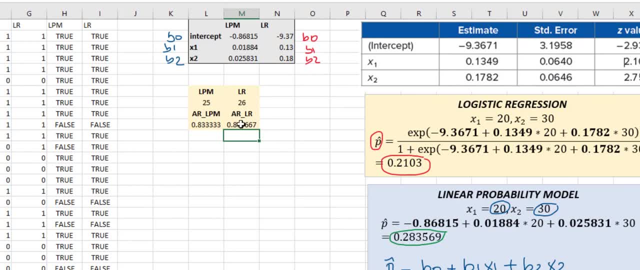 performs better than linear probability model, since the accuracy rate for logistic regression is greater than linear probability model. 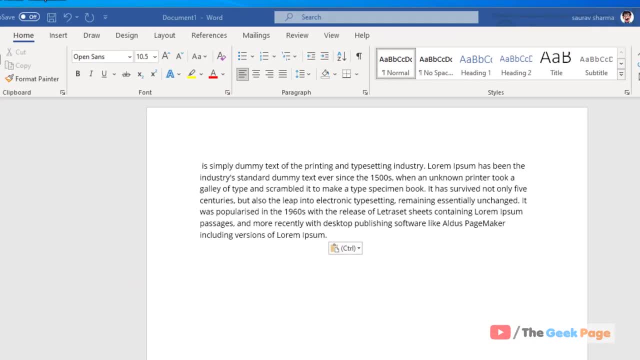 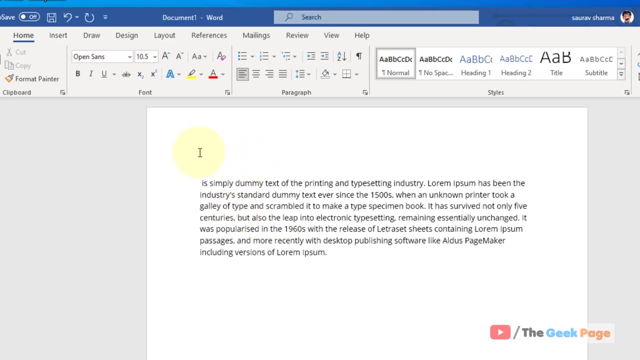 Hi guys, let's see how to insert a word count function in Microsoft Word. Let's say: this is your word document, So you want to insert a word count function here so that you can instantly check your word count every time you update your word.